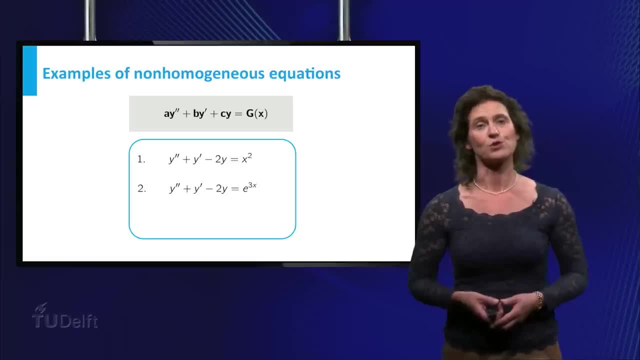 y. double prime plus y, prime minus 2 times y equals e to the power 3 times x. Then the equation is a non-homogeneous linear differential equation with constant coefficients, and y'' plus y' minus 2 times y equals the sine of x. 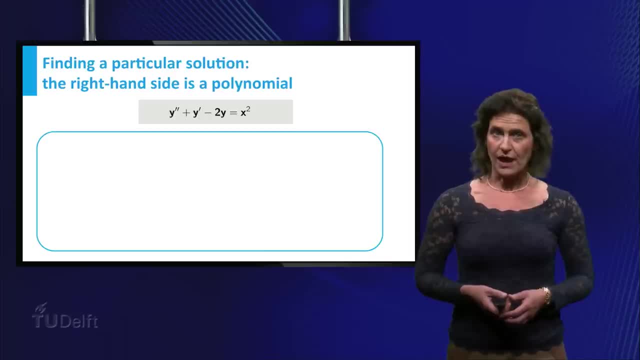 To solve a non-homogeneous differential equation, you have to go through several steps. One of them is to find a particular solution of the equation. Let's focus on this step. in the first example you just saw, Take a closer look at the form of the function of the right-hand side of the equation. 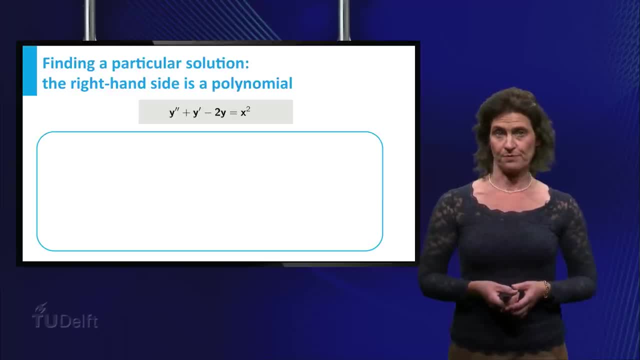 The right-hand side is a polynomial of degree 2.. A general polynomial of degree 2 is of the form: a times x squared plus b times x plus c for some real numbers, a, b and c. Let's try what happens when we take such a function as our guess for the solution y. 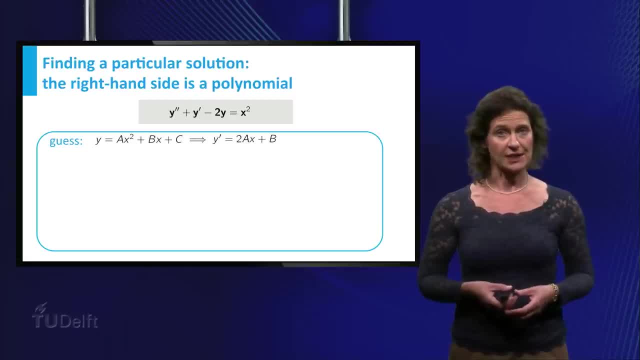 Then the derivative function of the function a times x, squared plus b times x plus c is the derivative of y equals 2 times a times x plus b, and the second derivative of y equals 2 times a. If this function were a solution of our differential equation, it should satisfy the equation in. 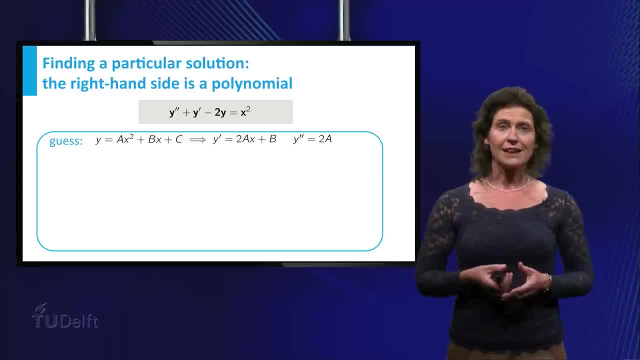 the grey box on the slide, Plugging in the expressions for y' and y', we find that 2 times a plus 2 times a, times x plus b minus 2 times a, times x squared, plus b, times x plus c equals x squared. 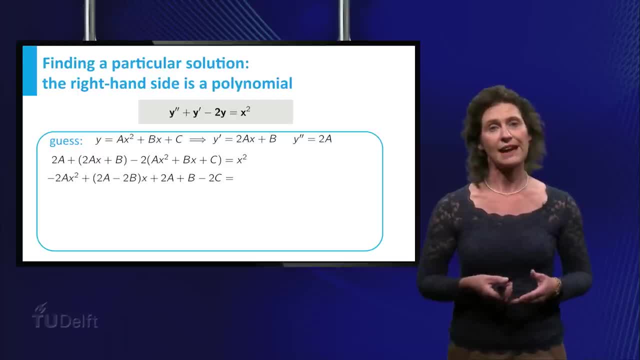 Rearranging the left-hand side gives: minus 2a times x squared, plus 2a minus 2b, times x plus 2a plus b minus 2c, The function on the left-hand side and the function x squared are equal to 2a minus 2b. 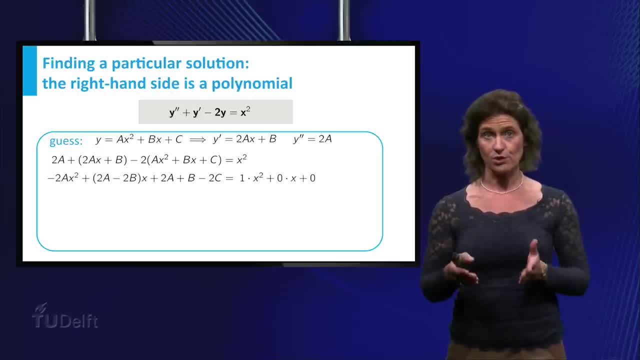 minus 2c. The brushstrokes for the right-hand side are also equal if, and only if, the coefficients of the powers of x are identical. Thus, if in the rewritten equation the left-hand side equals 1 times x squared plus 0 times,